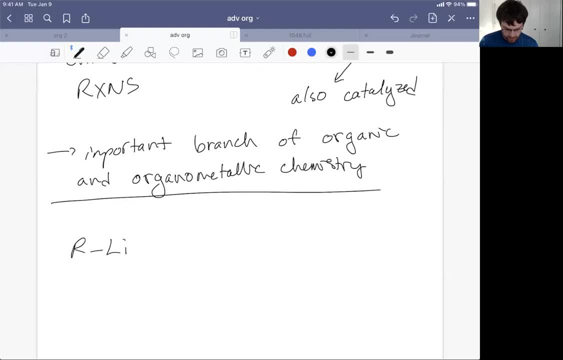 other classes there's. I'm going to start with lithium. I know it's not a transition metal And I'm going to abbreviate transition metals as TM for a while, And so transition means between kind of the main blocks of the periodic table. 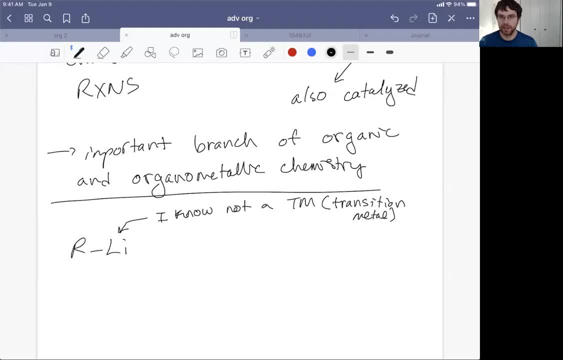 that bridge from the first two groups to the back, you know, the other three through eight, As we typically would say. there's that sort of kind of bridge between the two. Those are the transition metals. So lithium would not be one, But I like to remind us that we've been studying. 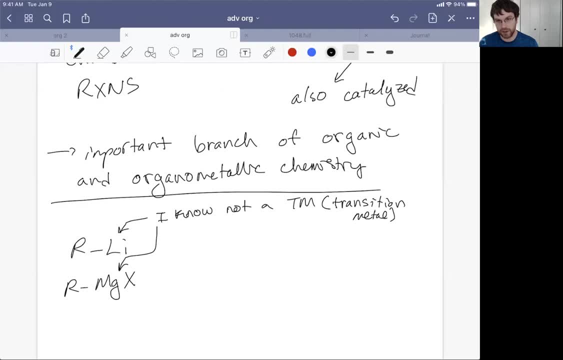 metal mediated reactions, So our organolithiums and our organomagnesium compounds. these are nice starting points, even though they're not transition metals. So both of these are not transition metals, but both have been used as good nucleophile. 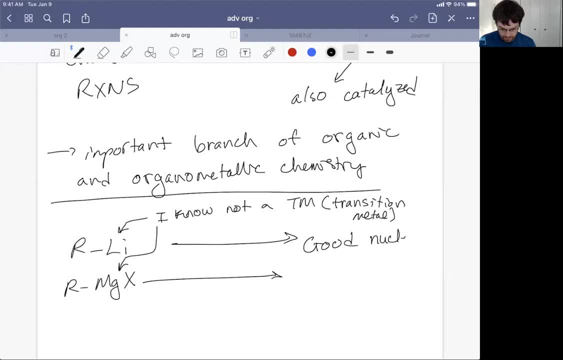 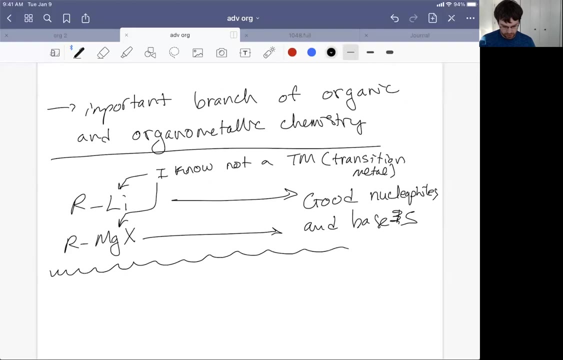 nucleophiles and bases And that's sort of to prime us for when we actually do look at our organometallic compounds, And so one that we saw actually in organic chemistry. two was the Gilman reagents. These are sort of these are like Grignard reagents. 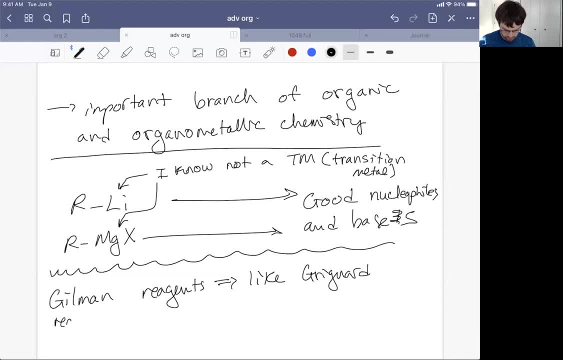 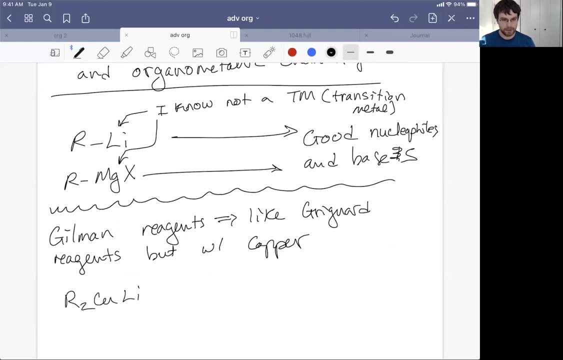 And they're all made of copper. So we'll take a look at that. next time we're going to talk about the process, But with copper. OK that we would say they were R2C, uLi And so Cu. now we have copper. 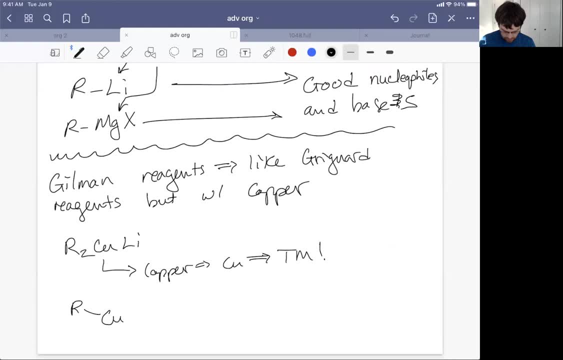 Now, another way of thinking about these was having R groups attached to the Cu. then the Cu would be overall negative, one charged, and so that would then be countered by a lithium plus. So the lithium is sort of a counter ion here. It's a counter ion to the copper complex. 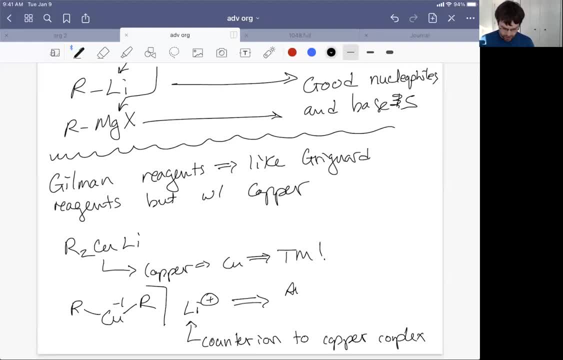 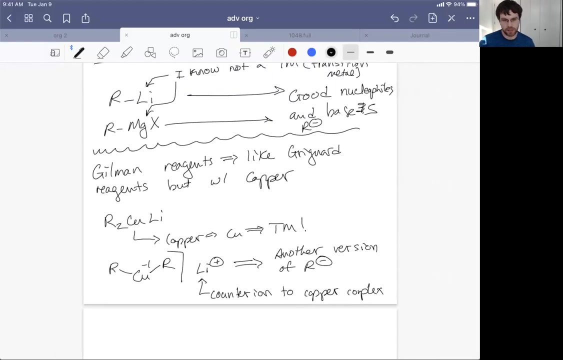 But this is now another version of R minus. R minus like our good nucleophiles and bases. the R minus is from the Grignard reagents and the organolithiums. Okay, sorry, I just went off screen there. I'm going to just take this out a little bit so I can keep going. 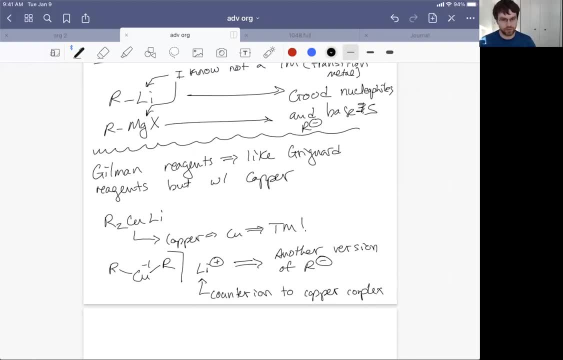 So with that in mind, we can start to think about how these things actually sort of work. I mean, a good starting place is to think when R is attached to a metal, Where R is some sort of carbon species, we have a delta plus on the R and a delta minus. 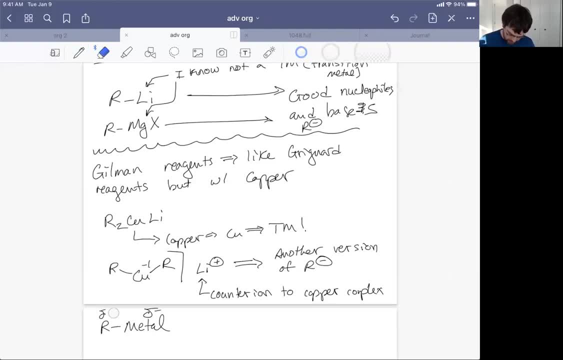 Oh gosh, excuse me, a delta minus on the carbon and a delta plus on the metal. Sorry about that. Sorry about that. I missed the whole point. Okay so, delta minus on the R group and delta plus on the metal. 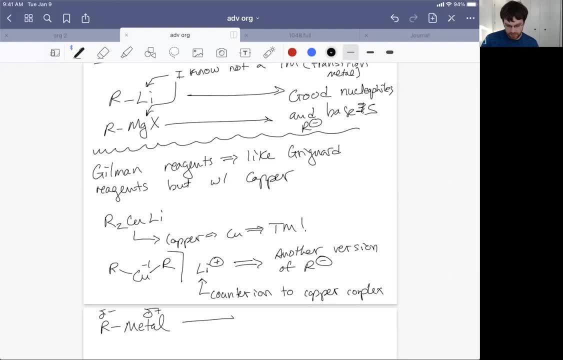 That is, the metal is much more electropositive than the carbon, And what I've tried to kind of hint at is that it's helpful to think about R minus being countered by some metal. But the equilibrium of this sort of covalent bond with the metal to an ionic bond sort of depends upon the metal that's actually being used. 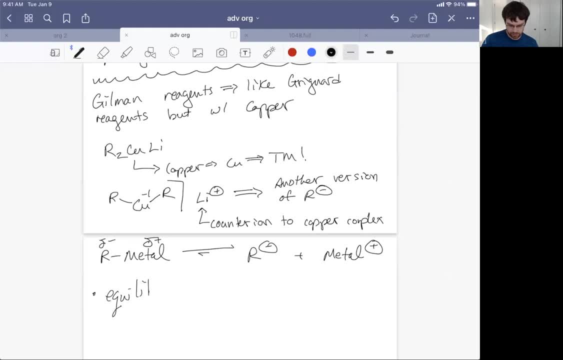 okay, so, um, what's cool about metal mediated and metal catalyzed reactions is that you start to get to some different reactivities, so i want to just remind us of some possible scenarios. 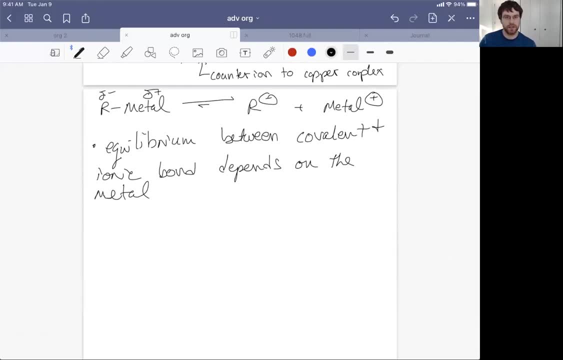 for when we take our our metal and we react it with um a, an alpha beta unsaturated carbonyl, like a cyclohexenone. so let's go ahead and take cyclohexenone and we're going to react it with R attached to some metal, and what i'm, what i want to do, is think about R minus engaging this. 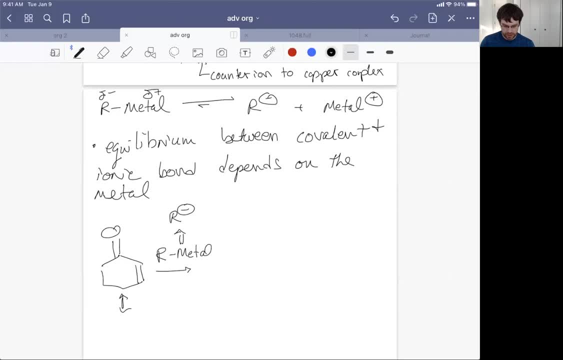 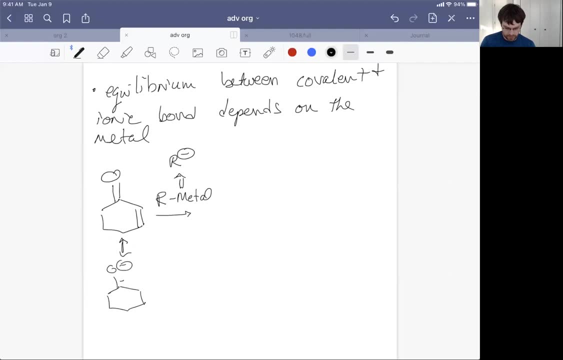 molecule. now there's a few ways to look at it. we could have the typical resonance structure of a carbonyl, where we have a negative charge on the oxygen atom and a positive charge on the carbon atom and a positive charge on the oxygen atom and a positive charge on the carbon atom, and 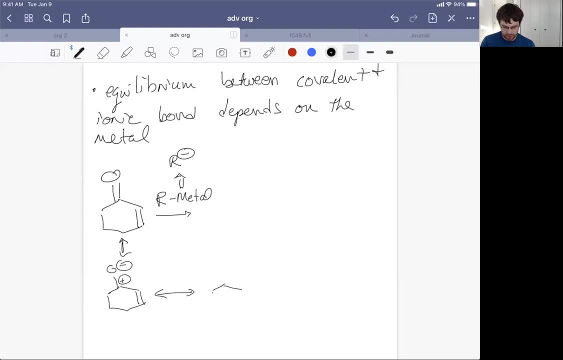 Adam, that's actually that actually could be further drawn as an enolate resonance structure with a positive charge at the beta position. So now we have an R minus that can attack the carbonyl carbon, or the beta carbon We call the carbonyl carbon, the one addition to the. 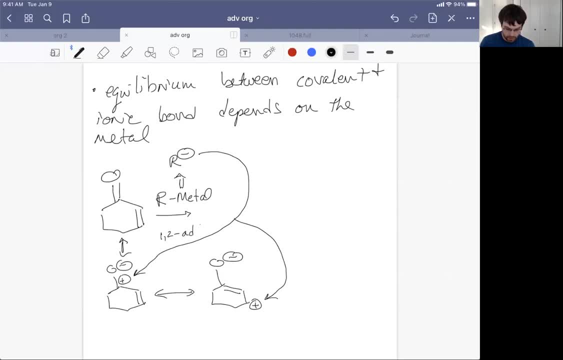 carbonyl carbon, this first resonance structure as our one two addition product, And then when we add to the beta position, it's our one four addition product. And the one four addition product would be like the what's called Michael reaction, from organic chemistry too. Now 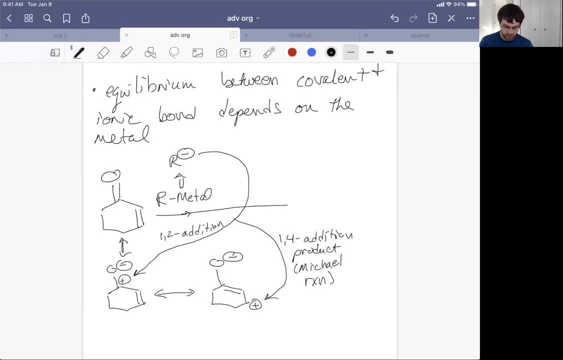 so what could happen is we could get then two products. If we add our R minus, we could get our one two products shown here plus our one four, our one four product shown here. Okay, So we have two modes of addition giving rise to two, I guess, alkoxide intermediates. that. 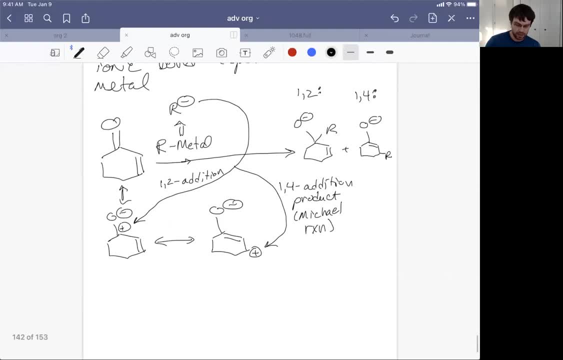 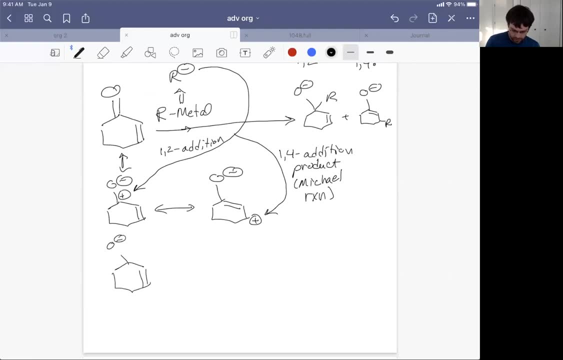 could react with H plus in a couple of ways And what we notice, and I'll go ahead and draw that. So if we react, let's go ahead and just be helpful. So if we have our, our alkoxide and we react it. 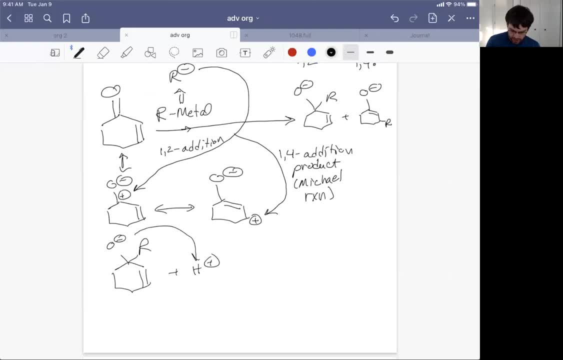 with H plus. in this case, the O minus just grabs the H plus, Negative to positive, neutralizing our molecule to give rise to an alcohol. In contrast, what happens is we could. we could certainly draw the O minus of our enolate, grabbing the H plus, but it would just undergo tautomerization. So I'm just going to show. 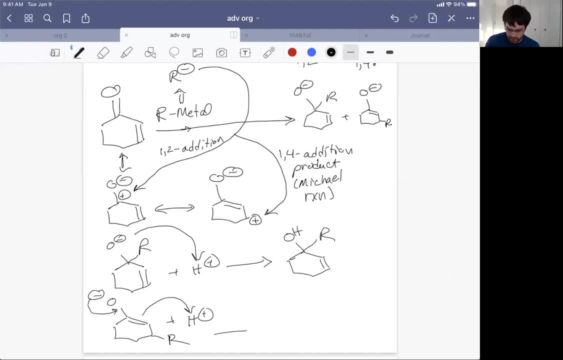 resonance reaching out and grabbing the H plus at the alpha position of our forming carbonyl To give rise to this species. It's not technically one four, unless you add the H to the oxygen and then tautomerize it. but let's just save a step So we can have our one two product and our one. 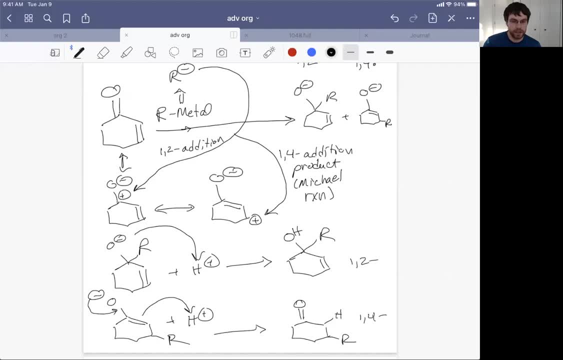 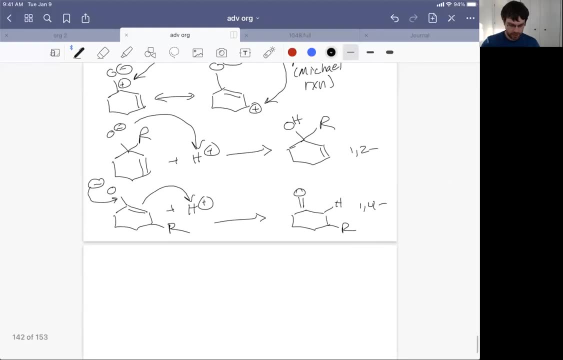 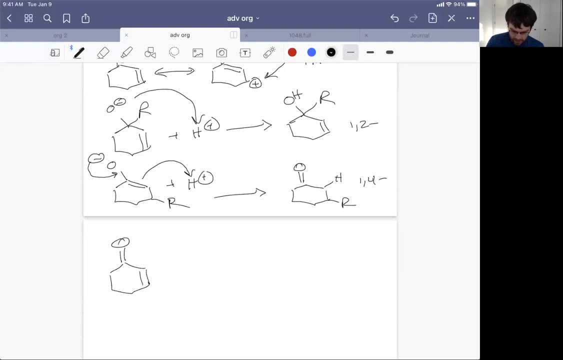 four products. Okay, Now there's a pretty cool experiment that you can do. You can take out an alpha beta unsaturated carbonyl and add to it a few different metallic agents. So let's take a carbonyl and we're going to add an organolithium to it. If we do that, the outcome- and let's go. 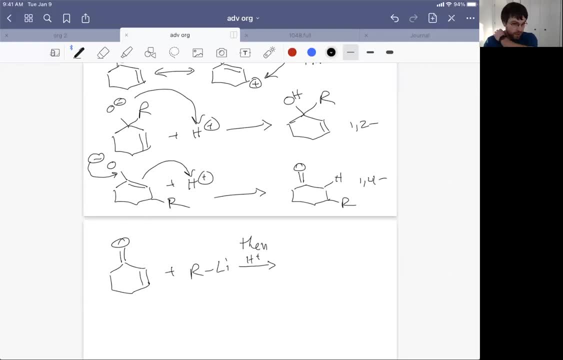 ahead and then follow with H plus. The outcome is as follows: For the most part, when you add an organolithium, you get one two addition. I'm going to write mostly: part of me wants to write only one two addition, but I don't think that's the case. 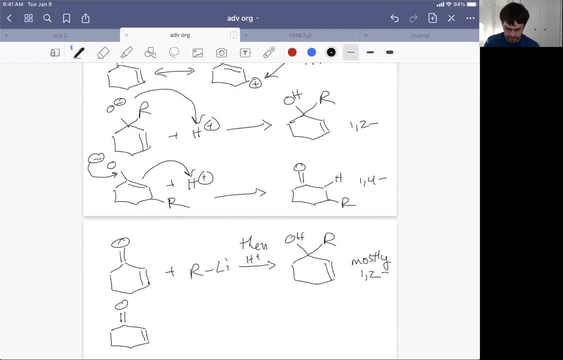 It's mostly one, two addition. Now that's in contrast to if we go to our old favorite, the Grignard reagent. everybody likes the Grignard reagent because it doesn't, like you know, ignite in the presence of moisture. It's much safer to handle that sort of thing. 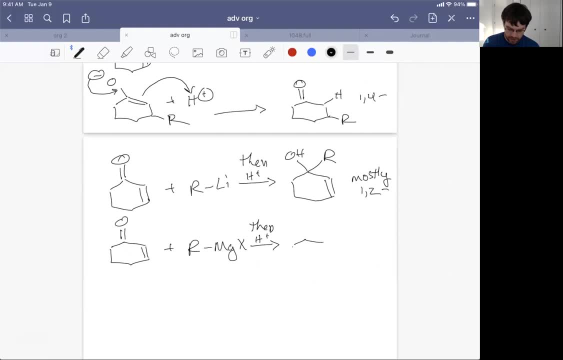 If you use a Grignard reagent for this reaction, though, you actually get a mixture of one, two and one four addition products. So you'd get your one two addition plus your one four addition products. Now, what's interesting about using a transition metal? that's kind of the goal of this chapter. 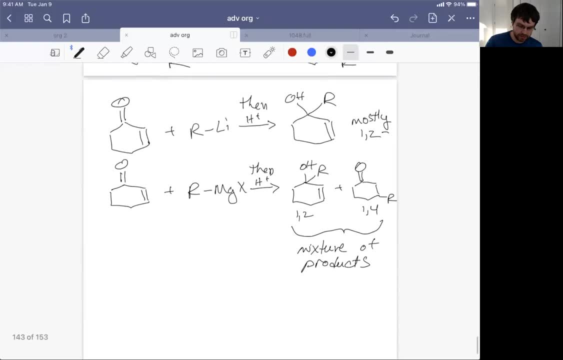 like, if we use copper, we actually get a different outcome altogether. Well, a different outcome from: yeah, yeah, sure enough, a good enough outcome. With our copper reagent, we actually get a different outcome altogether. Well, a different outcome from: 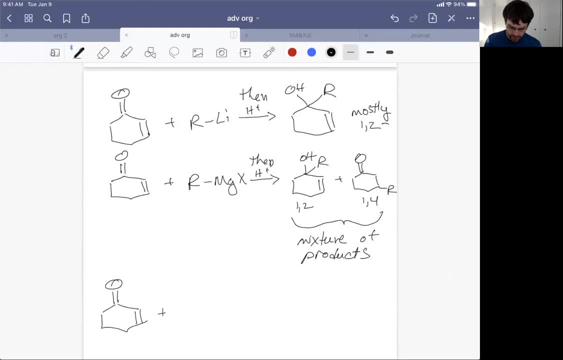 our Gilman reagent will selectively only get the one four addition product. So it actually diverges from both of the previous examples somewhat, And this is another depiction of a Gilman reagent. If you just write R2CuLi, that's fine as well, But if we have copper present, 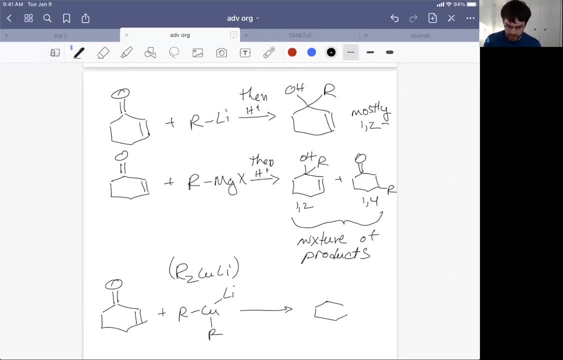 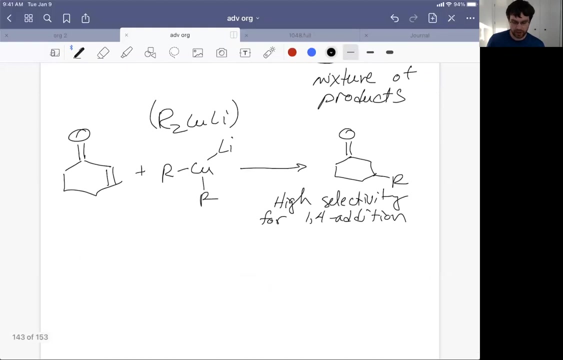 now we're going to exclusively get one four addition with high selectivity. So the transition metal actually allows us to kind of switch our selectivity and give different products in high yield, If we another way of getting this one four addition product. 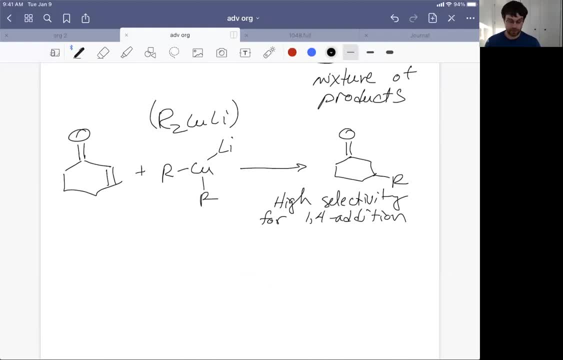 would have been to, you know, use the Grignard, do the Grignard reaction and then get it in low yields, as it would be then a mixture of products. So we're going to switch our selectivity and give different products. Okay, So what we have to do when studying transition metal mediated reactions? 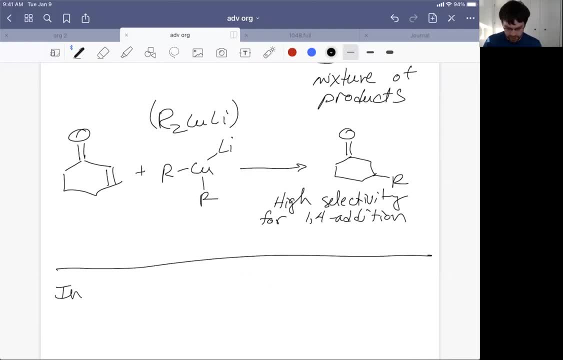 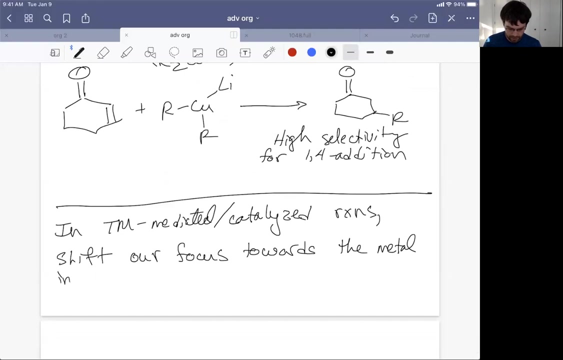 is we need to shift the focus. So, in transition metal mediated, as is the case above, or we're actually going to spend a lot of time with catalyzed reactions- We want to shift our focus towards the metal involved And we're going to ask questions like: for this metal, what's going on with its valence electrons? 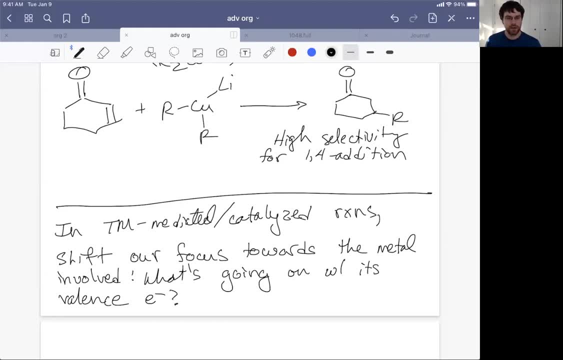 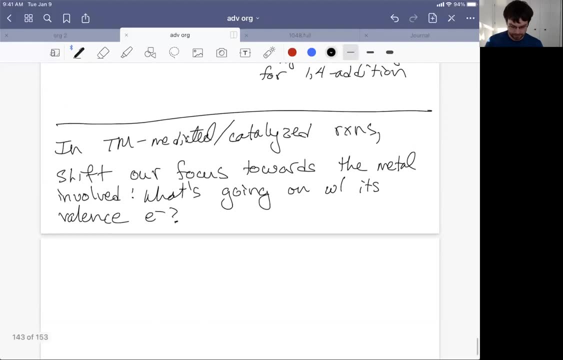 Okay, Now what we get is kind of an opportunity to introduce new things bonded to the metal. It's not really new things that can bond. I'm just going to write different things. So different things can bond to metals and the bonds can be ionic, covalent as a sigma bonds and covalent as pi bonds. 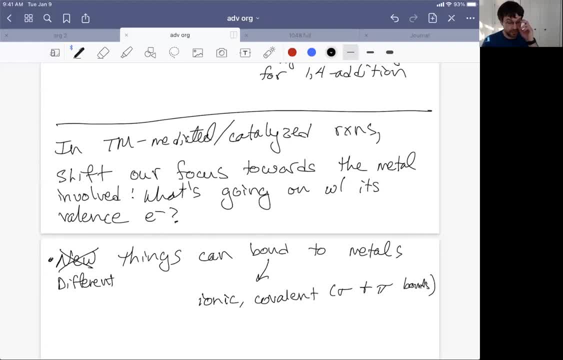 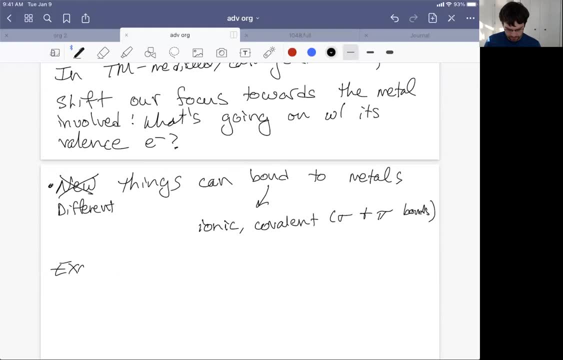 So we really get the entire bonding arsenal to many of these transition metals that we're going to study. So, for example, we could have a palladium complex- This is our transition metal- And the transition metal could be bonded to P, which is attached to three phenyl groups. 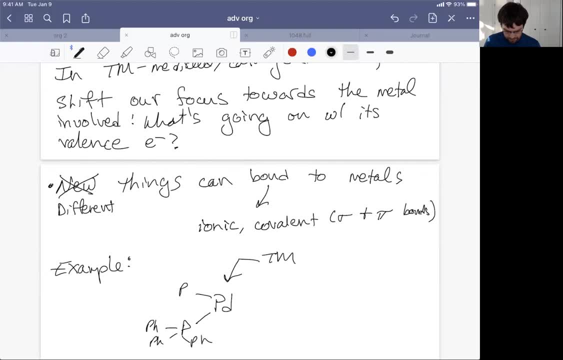 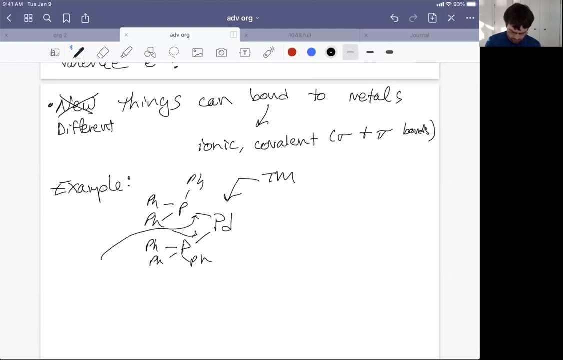 So P again is phosphorus. So we show a bond to the phosphorus atoms And then we show a bond to the copper, And then we show a bond to the copper, So it's a two electron sigma bond to phosphorus. But then we could also bond with the pi bond of a double bonded system. 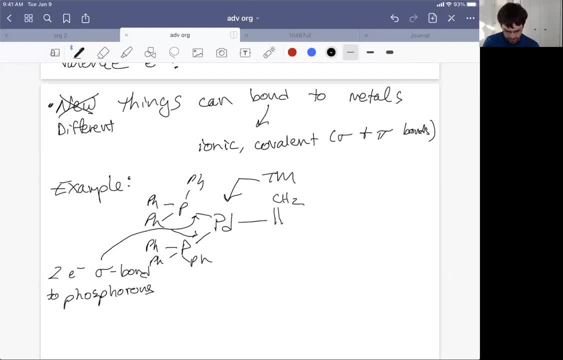 So I'm going to draw a line over to an alkene. That is something with a double bond between two CH2s, And I'm going to be very careful about my drawing just this first time. So I'm going to have the line from the palladium to the ethene. 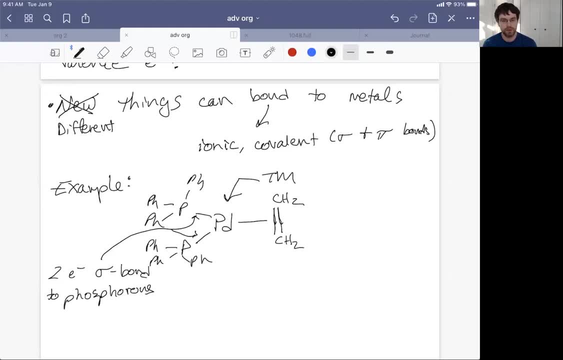 I'm going to have it just kind of bump right up into the electrons that are bonded between the two carbon atoms. So we have a carbon-carbon double bond And it's that bond that actually supplies two electrons from the pi bond. Okay, 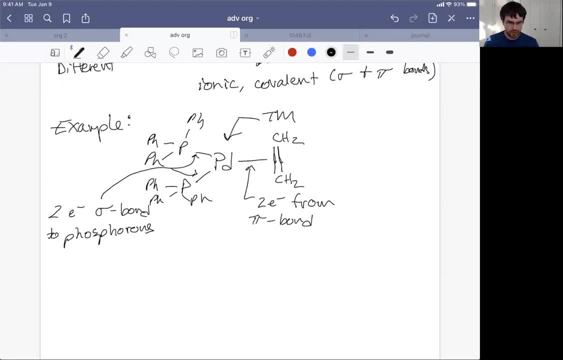 So what we say, then, is: palladium is attached to a bunch of non-metal atoms. It's actually attached to four non-metal atoms, And how is it attached? It's actually attached to a number of non-metal atoms, And how is it attached? 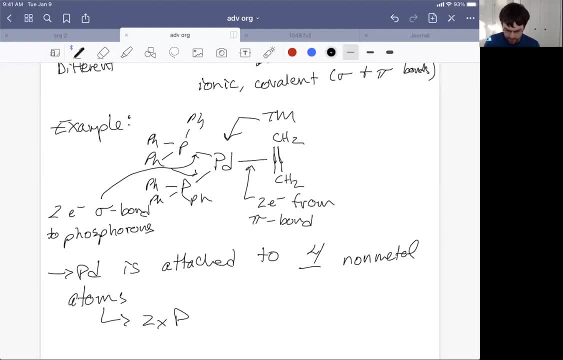 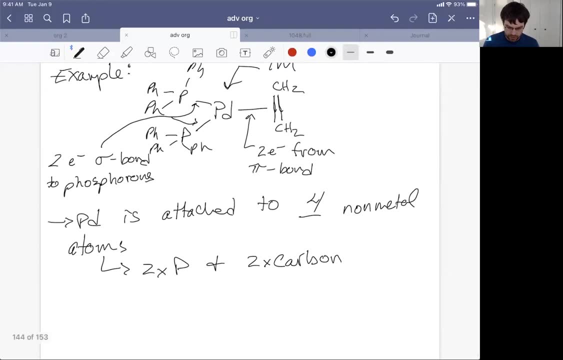 It is attached to two times phosphorus and two times carbon. Now the carbon one is kind of interesting, Because up here palladium forms a complex with the pi electrons on both carbons, And so we say that it's simultaneously attached to four non-metal atoms. 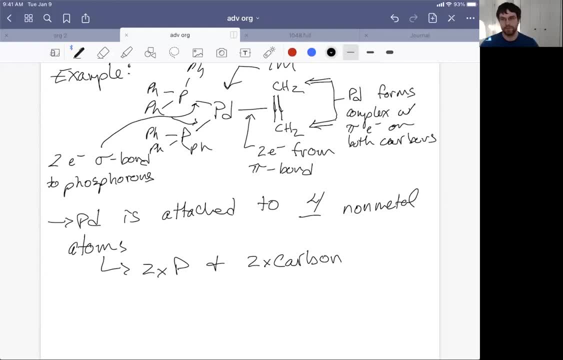 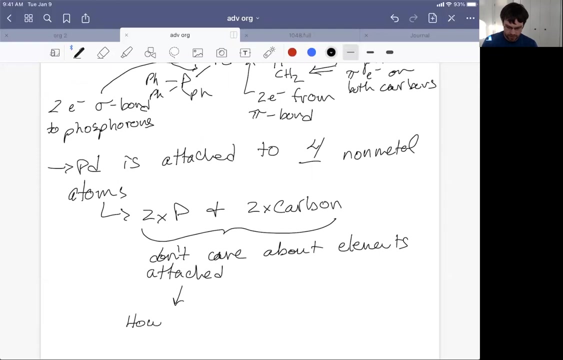 Two palladium and two carbon atoms. Now, what's sort of interesting about this is: I don't really care about the number of elements attached. Instead, I want to focus on how many electrons does each atom provide? And because these atoms, because these things that are attached to the transition metal, could be atoms or even bonds, I want to replace. 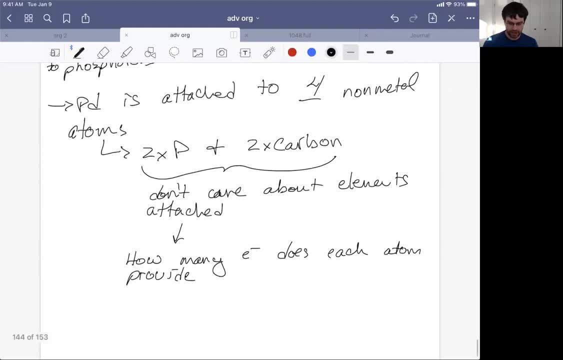 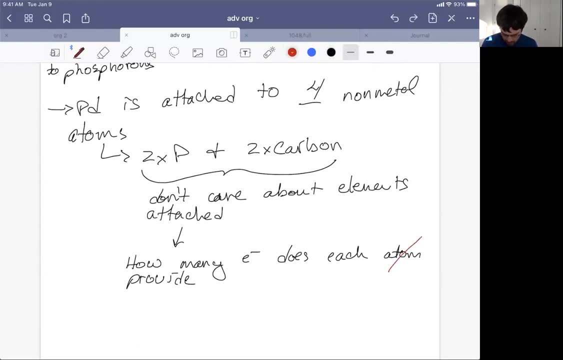 I want to be a little bit more general as to this. I want to be a little bit more general as to the type of things that can attach to my transition metal. I'm going to cross out the word atom over here. I'm going to cross it out in red so you can see it. 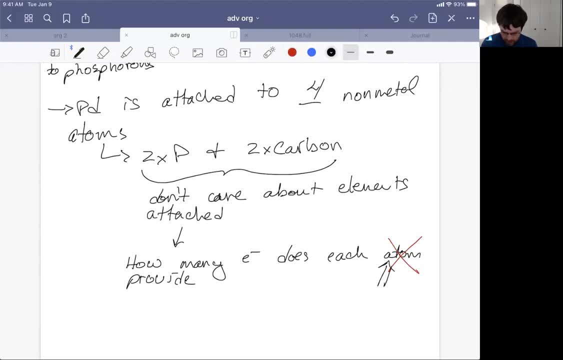 I'm going to cross out atom And I'm going to replace it with a better word, which is ligand- Ligand- Some people call it ligand, I don't really know. So, instead of focusing on the atoms that are attached to the transition metal, 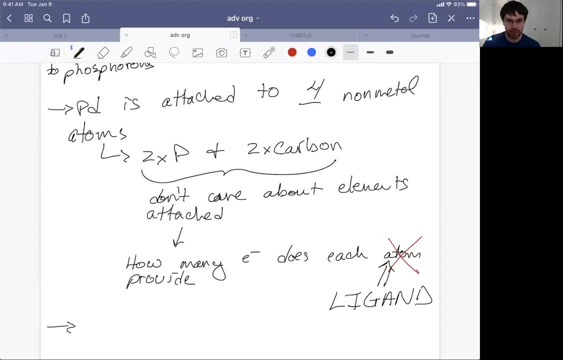 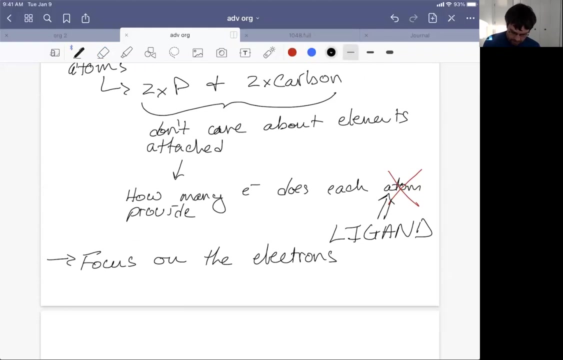 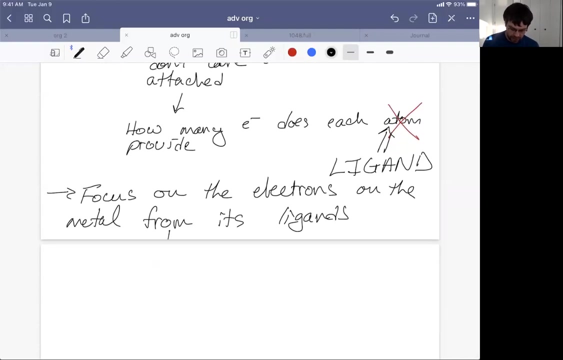 I want to focus on the electrons available to the metal, the transition metal, from the ligands. So I want to focus on the electrons from actually electrons on the metal, From Actually electrons From It's ligands. Okay, And it's this that actually controls. 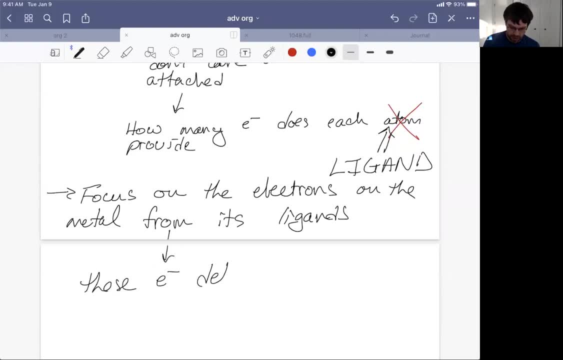 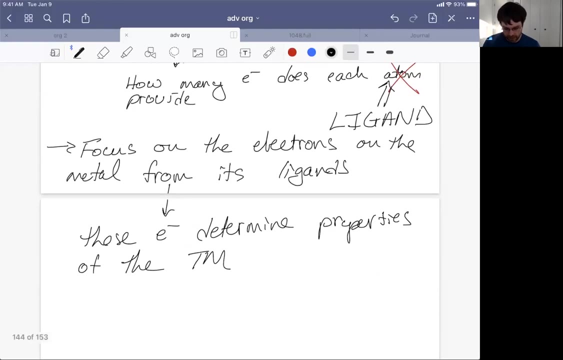 These electrons really determine the property Properties Of the transition metal. So that's pretty cool because that suggests that a transition metal can actually have Vastly different properties from another. a transition metal in a complex could have vastly different properties than the same transition metal the same palladium type of element. 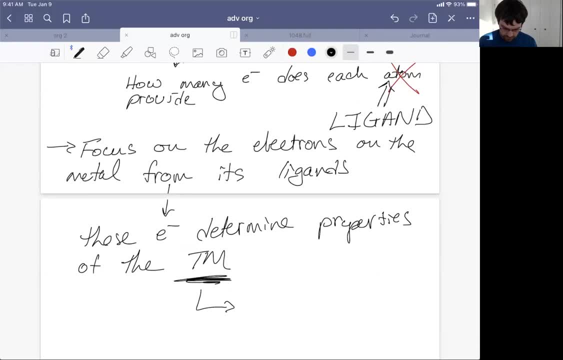 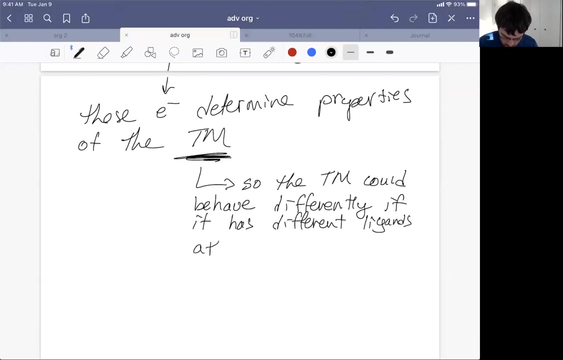 As long as it has different ligands attached to it. So the transition metal could behave differently If It has different ligands attached. Okay, In this case, if you've got P, And then I'm going to write just PH three over here like this: 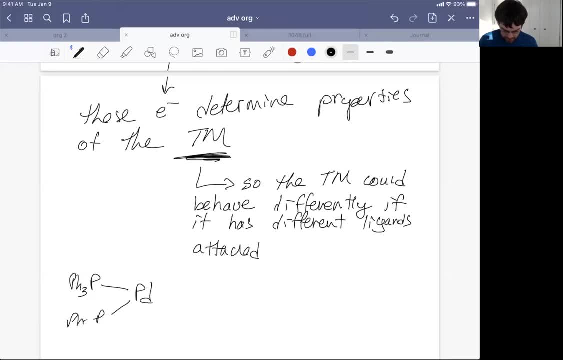 And that's attached to palladium. P, PH, three like this, And then we have our PI complex Two And ethene. We actually get a grand total of six electrons from the ligands. Now I don't want to spend too much time on this. 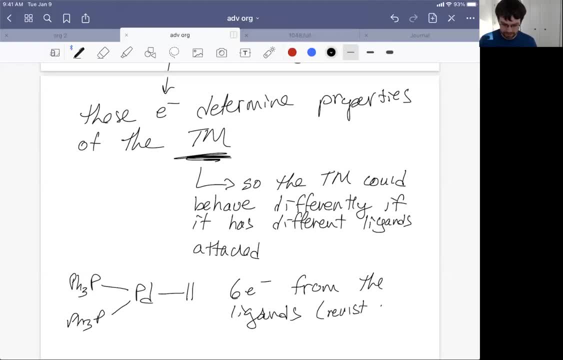 We will revisit in a later lecture. But the fact that we have Six electrons from the ligands means that this Complex is going to behave differently than if we had Four palladium, Four phosphorus ligands attached to our palladium. 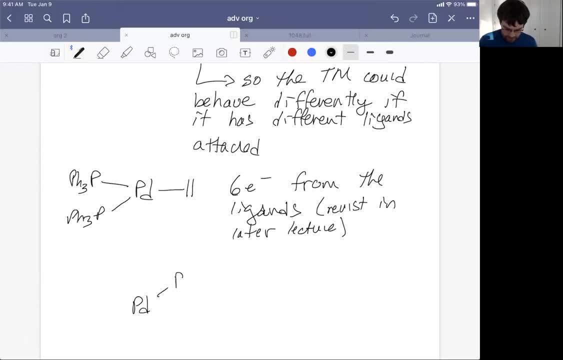 For example, if we had a palladium Attached to PPH three here, PPH three, here, PPH three, And it's the phosphorus, That's the attaching Adam. Just on that phosphorus, We have four Phenyl groups around it. 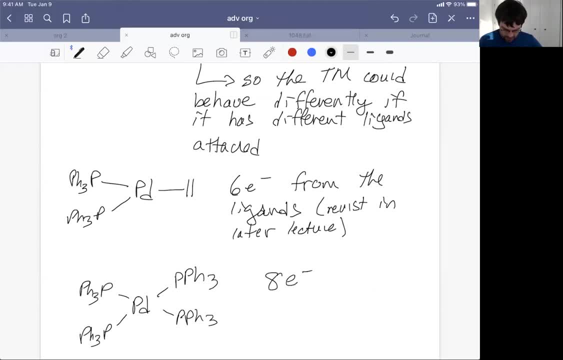 We would say that in this case we actually get Eight electrons From The ligands. And again, don't worry about where I'm getting the six and the eight, Just worry that the, the metal complexes are different And the electrons from the ligands are different. 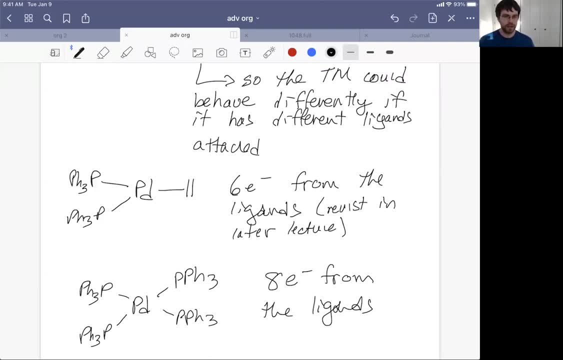 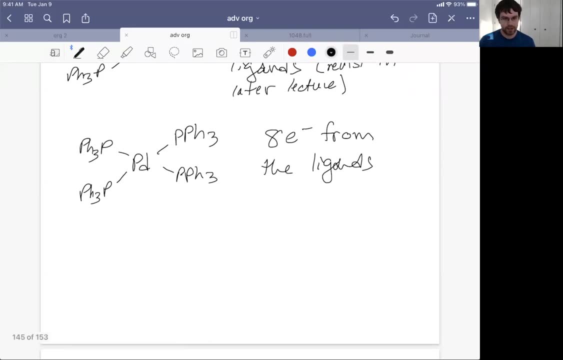 Now, before we move into- and I think counting electrons around the transition metals is Some of the more important things we'll get from this unit- before we get into that, Let's just look at some Conventions. So conventions when studying. 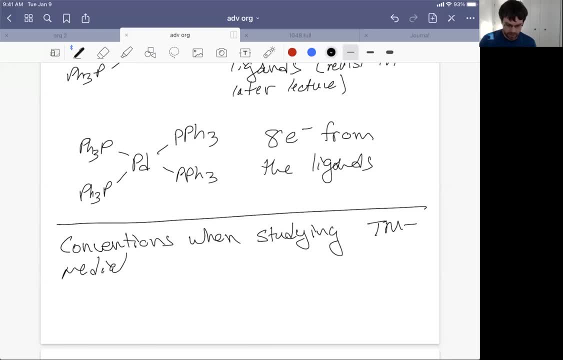 Transition metal, Mediated Or actually just transition metal complexes. Okay, The the one that took me a little while to wrap my head around Was there are no formal charges used. Okay. So, for example, if we had- let's say we have- palladium, 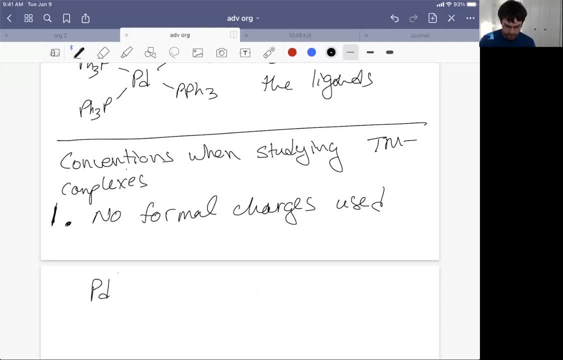 Two plus it's in the plus two oxidation state And that that positive two indicates You know you could see a plus and a minus Between The two oxidation states And that That positive two indicates That there's a plus charge. 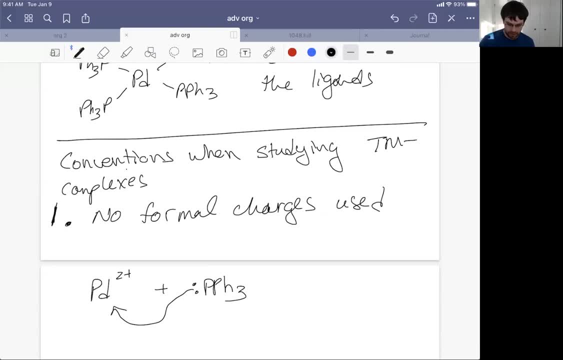 Between The PPH three, which we've seen is a pretty good ligand. We could have those interact. Now, typically, If we had some sort of electrophile, Just general electrophile, And we let the PPH three react with it, We would get 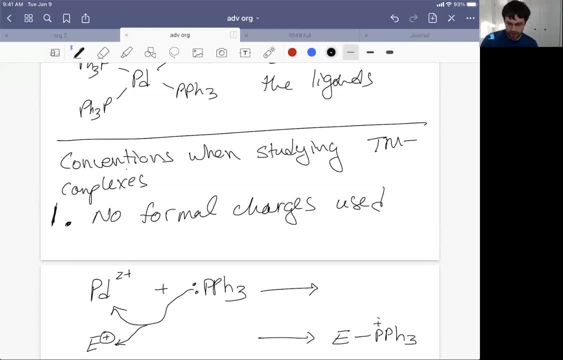 Electrophile being neutral, and then PPH. three, phosphorus is in the same group of the periodic table- is nitrogen. We put a A plus Charge on the phosphorus And then we would neutralize the. We would neutralize the plus one oxidate or the plus one charge of the. 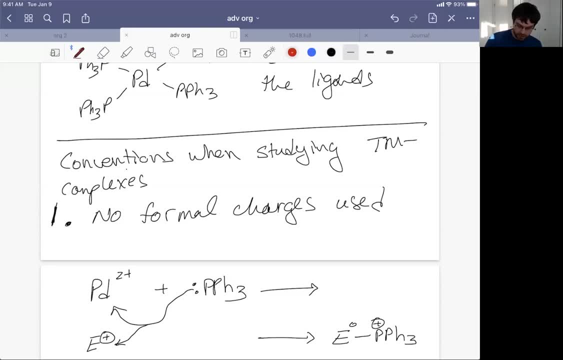 electrophile in this case. This is not what we do for transition metals. Okay, That may work with like a carbon based electrophile, But what we do with transition metals is we write palladium two plus Bonded to PPH three. 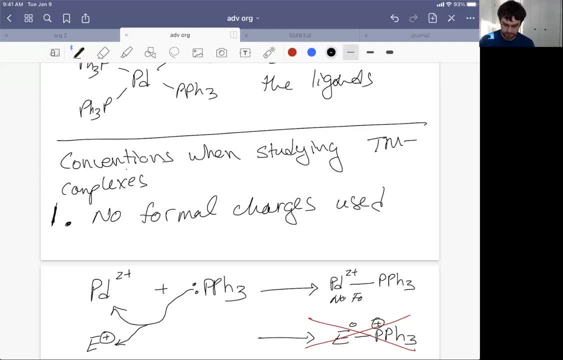 No formal charge. So now, even though the Palladium- Excuse me- even though the triphenyl phosphine, The phosphorus with three phenyl groups around it, now has four Sigma bonds, We don't write any formal charges on it. 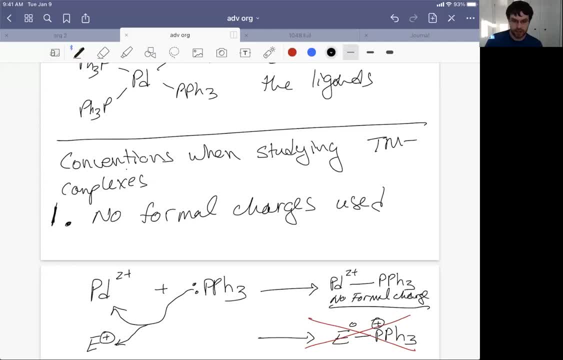 We just keep it as is, which includes the plus two oxidation state, And we just write the PPH three bonded And we just kind of get used to it. Notice I didn't decrease the charge on palladium By one, which is what I did with the generic electrophile. 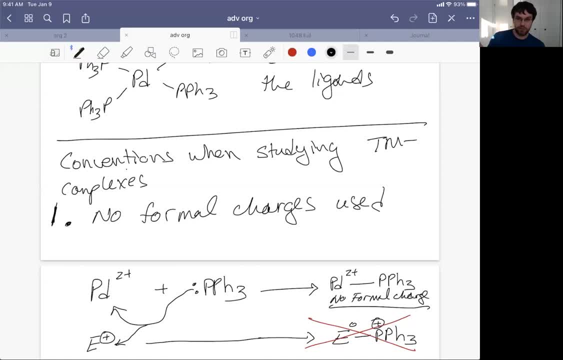 Instead, I just wrote Palladium two plus. still, it's as if the oxidation state Was not affected. Okay, Now what we have to do is we need to be careful when we let ligands bond To our metals, When we let our non-metal atoms of our ligands bond to our metals at all. 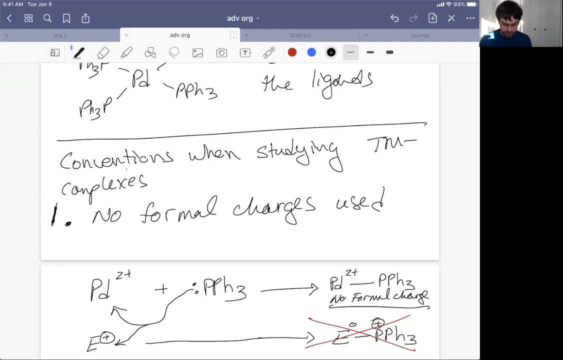 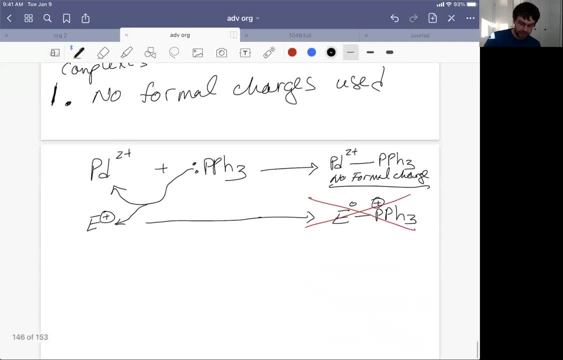 So okay. So so far you're like: okay, I guess I can get used to it. The palladium plus two Keeps its oxidation state And you just draw a line between it and the triphenyl phosphine. But what if we have palladium two plus? 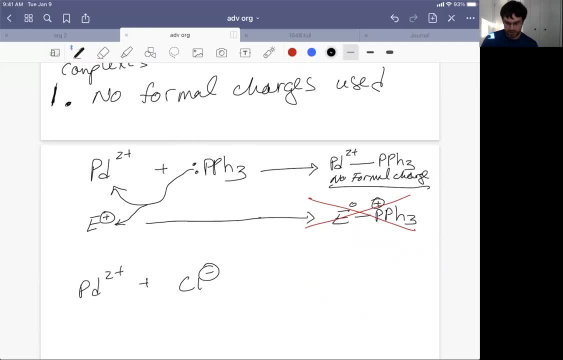 Reacting with A CL minus. CL minus is also Often seen as a ligand. We really want to draw a curly arrows, right? We really want to draw a curly arrows to show the formation of palladium chloride, And then let's just have the palladium neutral. 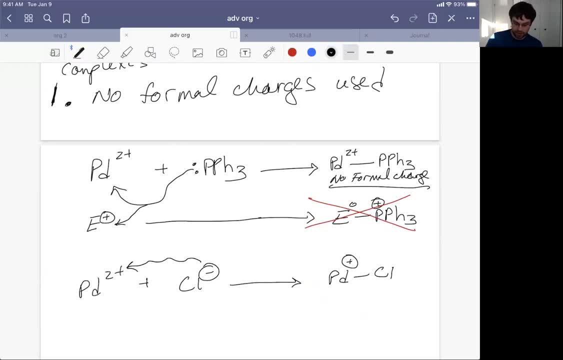 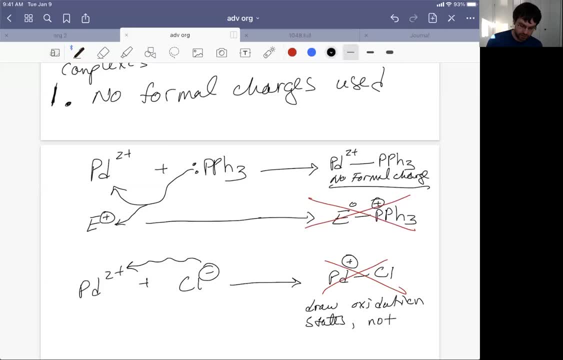 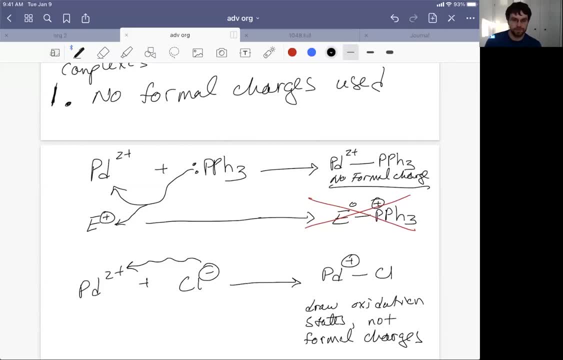 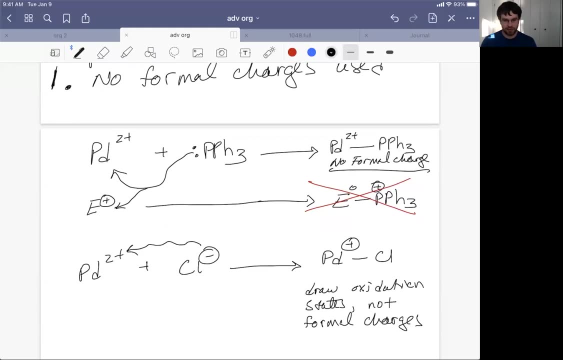 Well, yeah, The chlorine doesn't have a charge. So What we have to consider when we're doing this is This: there's not like a really good kind of Common, common set of rules for just drawing these complex. I say that. 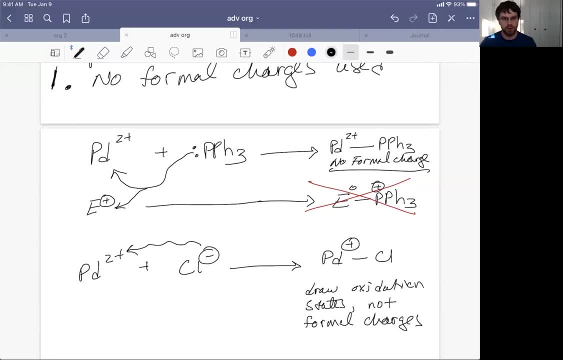 And I'm like: well, I'm thinking through all the rules, Well, the rules just don't really jive with what we, what we do with main group Of atoms like chlorine, Phosphor, carbon, phosphorus, chlorine, those sorts of things. 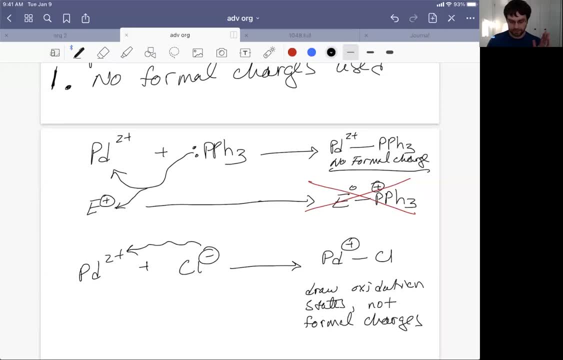 As soon as we introduced transition metals, We have to kind of We have to kind of follow a new set of rules. Let's just immediately move into Some, some, some, some more kind of different ways of thinking about this. Okay, 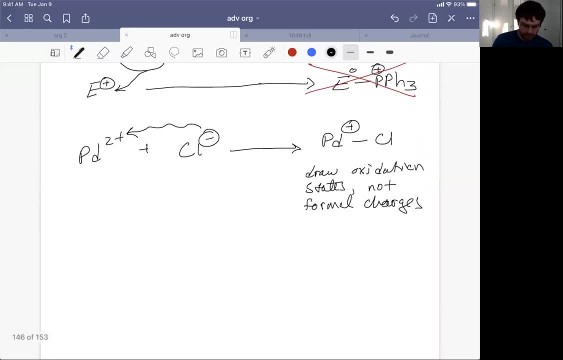 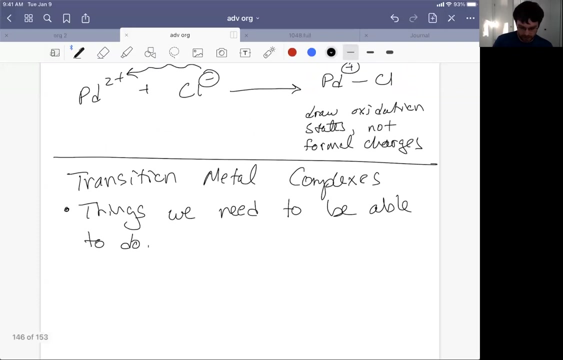 So let me just first of all cover what we need to know about our transition metal complexes. Okay, Okay, Okay, Okay, Okay, Okay. Well, the first thing, These are Things we should be able to do. Number one: 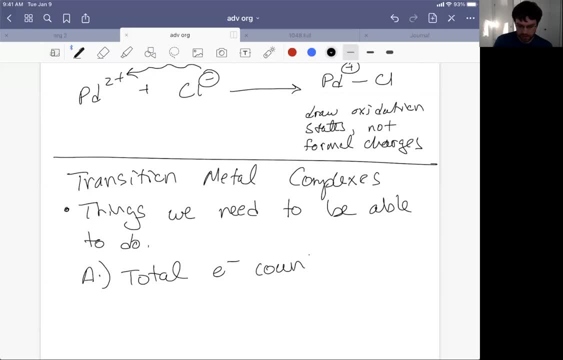 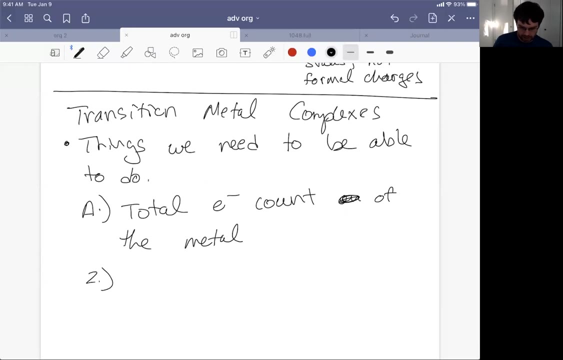 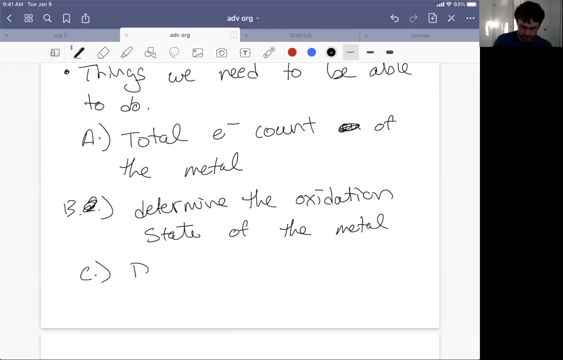 We need to be able to determine the total electron count On, Or of the metal Number two, we should be able to determine the oxidation state of the metal. I guess B determine the oxidation state of the metal. Okay, and then C we want to determine. 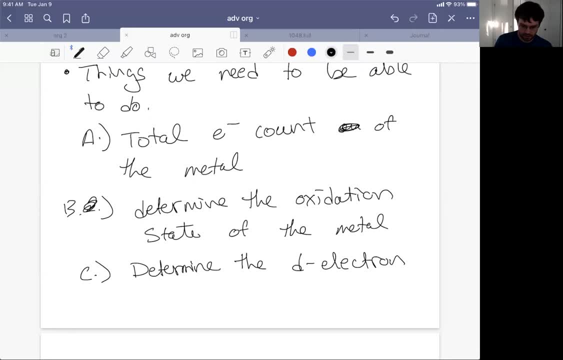 the D electron count of the metal. Okay, So what we'll do is we'll spend some time looking at how to determine each of these things. So something that's really helpful for getting into this is to look at what's called the 18-electron rule. 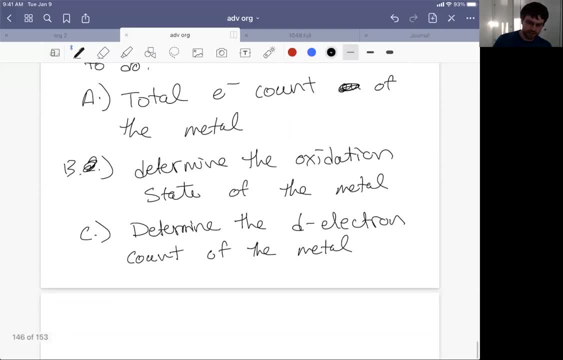 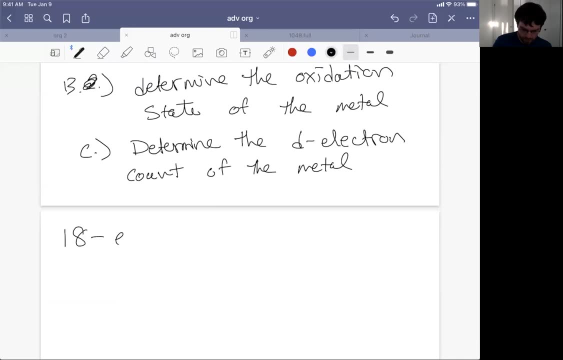 And so the 18-electron rule is kind of like the octet rule, but for transition metals. OK, so the 18-electron rule. We'll touch on this before we break for this lecture. The 18-electron rule says that thermodynamically stable, 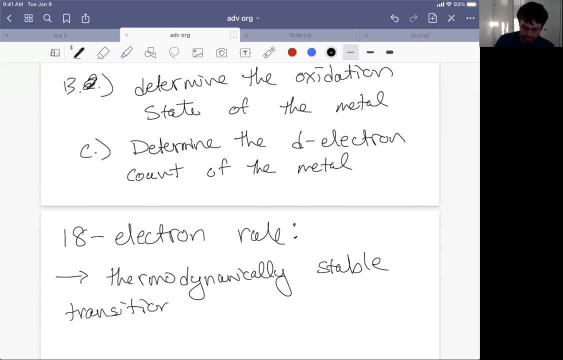 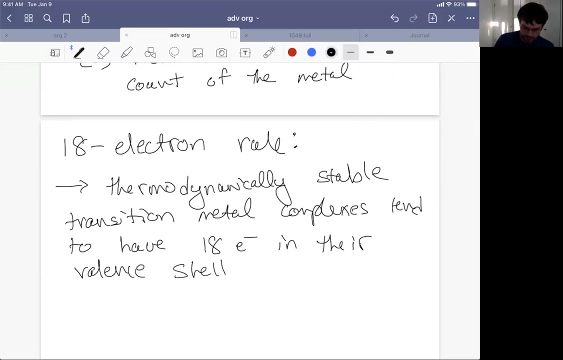 transition metal complexes Tend to have 18 electrons in their valence shell. Now, as I indicated, this is like a transition metals octet rule, except instead of 8 for the octet rule we have 10, an extra. 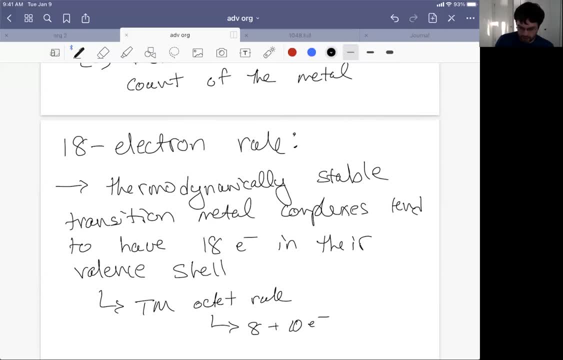 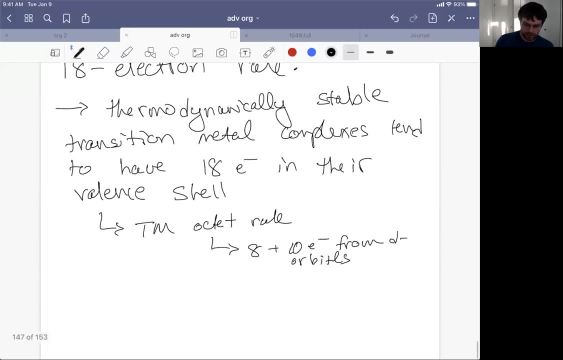 OK, OK, OK, OK, OK. 10 electrons from the d orbitals. So said another way, if you recall, for each shell around a nucleus- And these are the shelves that we put our orbitals in- For each shell around a nucleus, beyond the second shell. 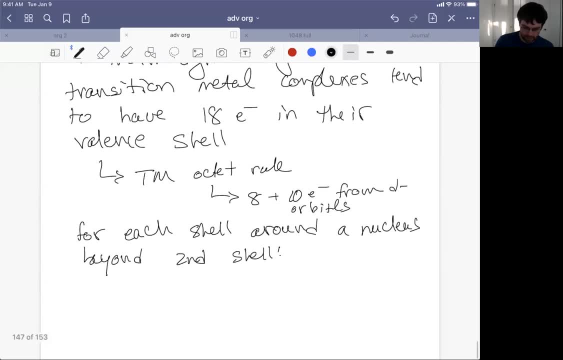 we have um one times an S orbital, So the S orbital can hold two electrons. We actually have three P orbitals, all orthogonal to each other: PX, PY and PZ. So we have three of those. We have three orbitals. We can hold six electrons total, So two plus six. there is our. 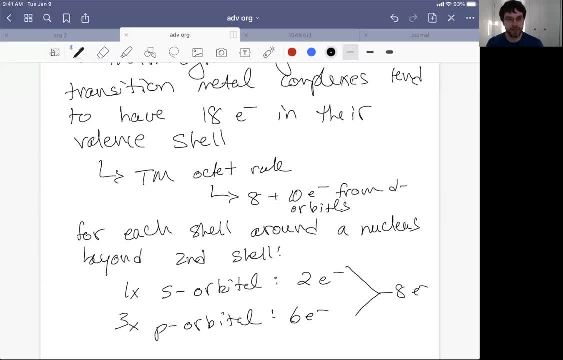 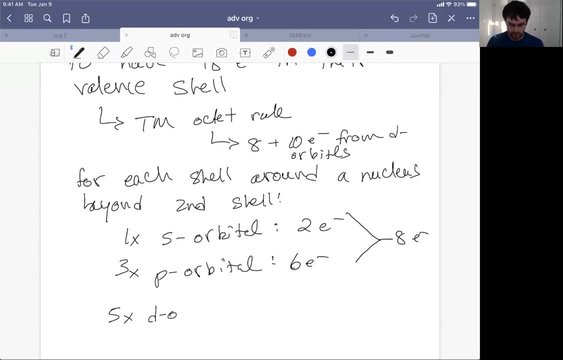 eight electrons of the octet. Now what we can do additionally is consider our five D orbitals. If you've taken descriptive, you know these have some interesting shapes. but now five times two is 10 electrons, So we get eight plus 10. 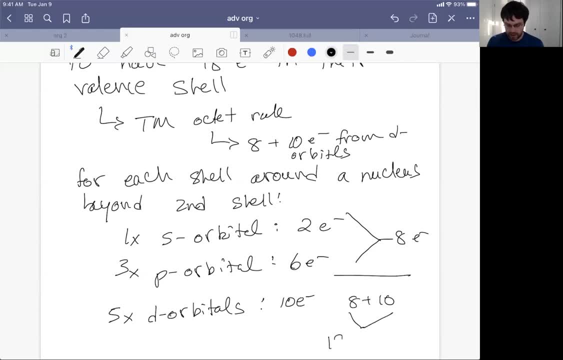 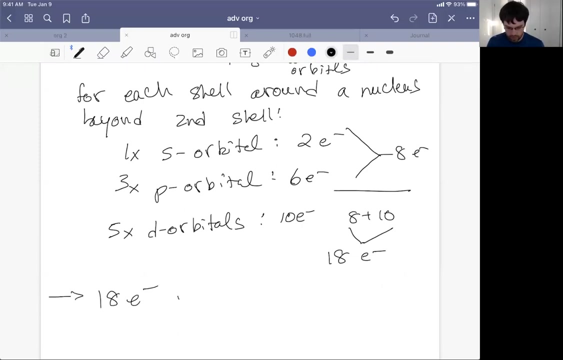 equals 18 electrons, And because our transition metals are all beyond row three, they actually do Take advantage of their D orbitals quite a bit, allowing us to get up to um 18 electrons to fill a shell, Okay, So it turns out, though, that the 18 electron rule is helpful. 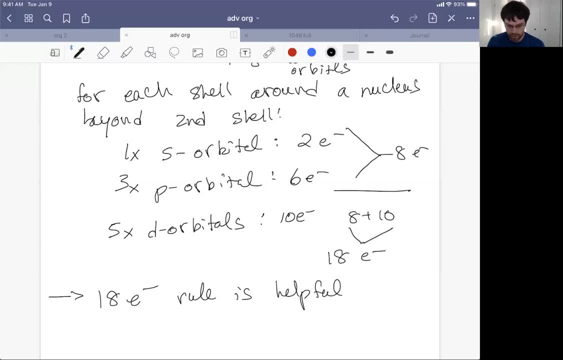 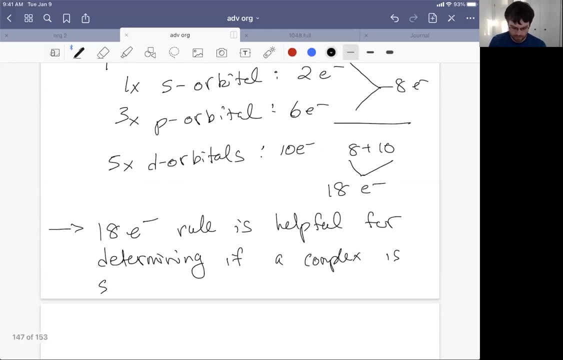 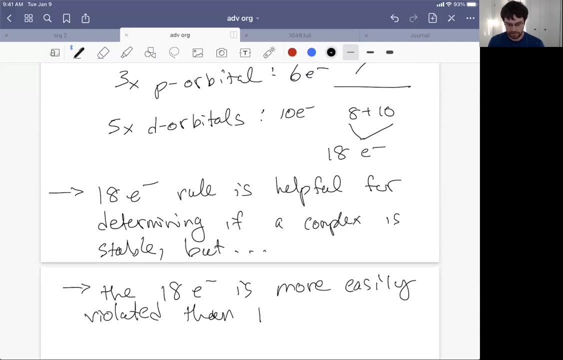 for determining if a complex is stable. So this is true, but dot, dot dot. the 18 electron rule is more easily violated than the octet rule. So you can break the 18 electron rule, but you can't break the octet rule. 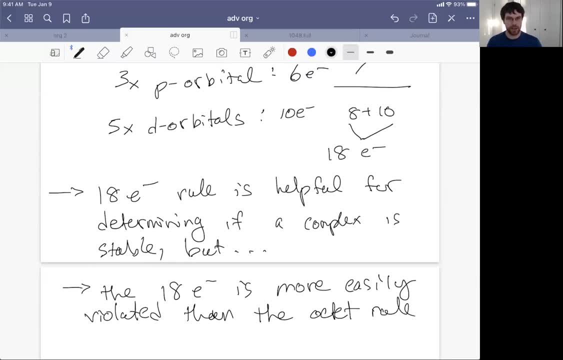 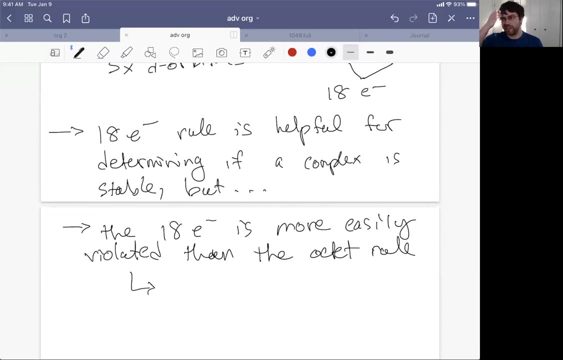 So you can break the 18 electron rule, but you can't break the octet rule, and you do so pretty easily just by like having stuff randomly fall off, And so you don't always, you don't always kind of go over the the 18 electron rule I can't think of. 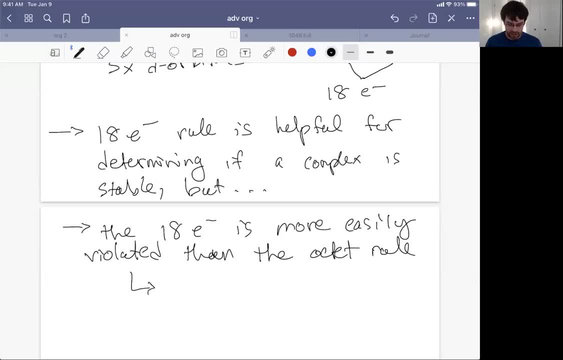 really any, any example off the top of my head, though I'm sure some exist. But by violate I mean you fall short or have less than 18 electrons. So that's common. It's common to have less than 18 electrons, much more common than it is to have. 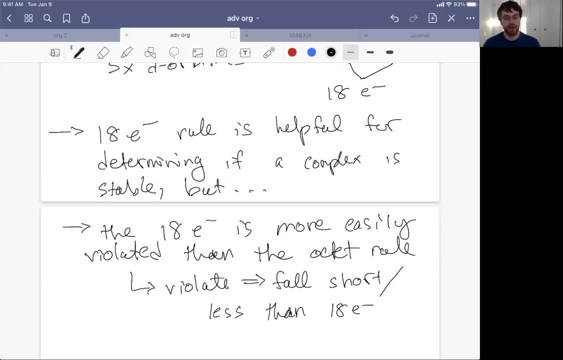 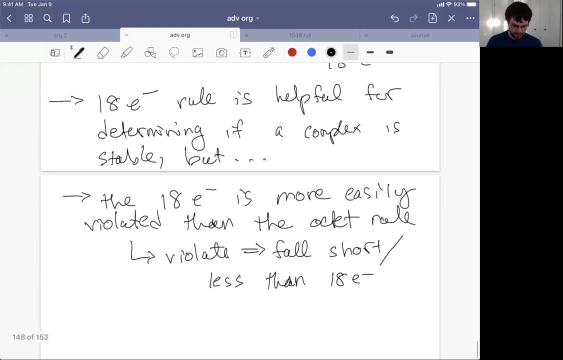 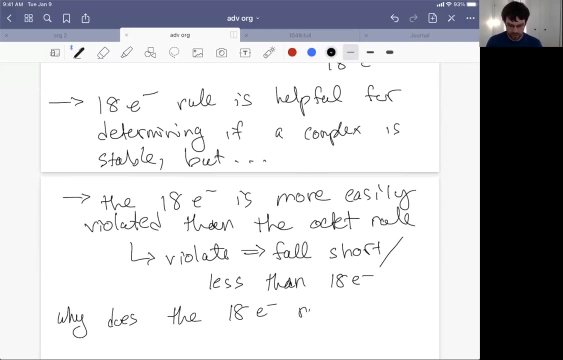 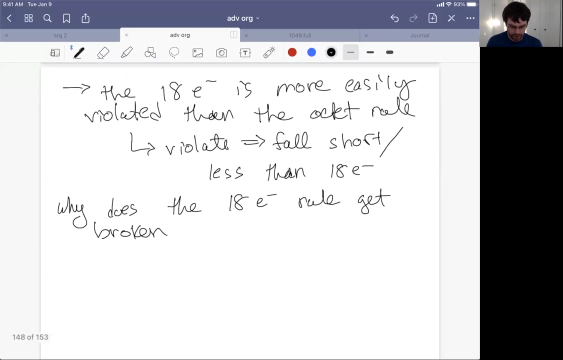 less than eight electrons for a typical main group. And the reason why is- we could ask that we could write that specifically- why does the 18 electron rule get broken? Okay, So why does the 18 electron rule get broken? Well, there's a lot of deep arguments as to why. 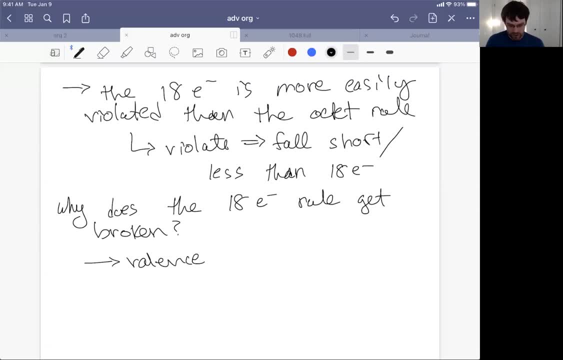 but generally we just could say that the valence shell that we're filling up to 18 electrons is far from the nucleus. It's far from the nucleus compared to the first and second shell. So it's farther away if we're in a row three element than it's the third shell. you know. 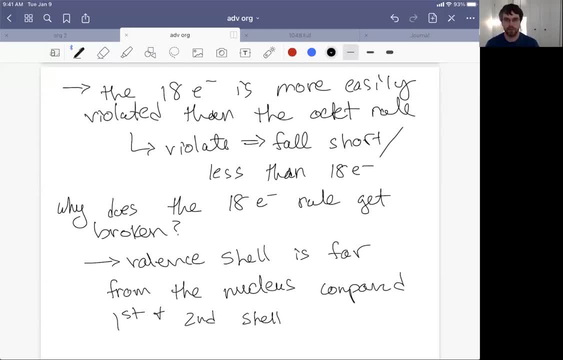 you keep going down the periodic table, you get further and further away from the nucleus. it's easier to break those rules, be off by a charge countering the nuclear charge. Now, the other thing that's important to realize is that with the octet rule we could kind of fit. 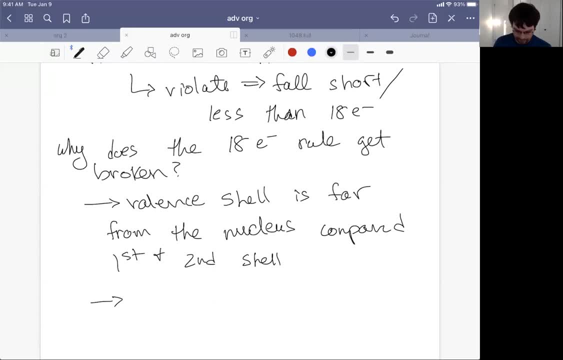 four things around a carbon atom to hit its octet. But fitting enough ligands on a metal to get to 18 electrons can be difficult, So it can be hard. So what we need to, we need to do, is need to do- is figure out how to determine how many electrons are on the transition metal. 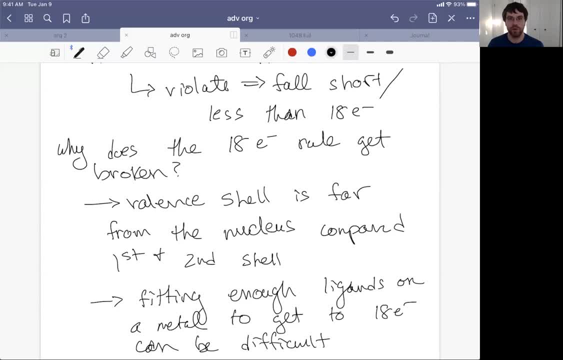 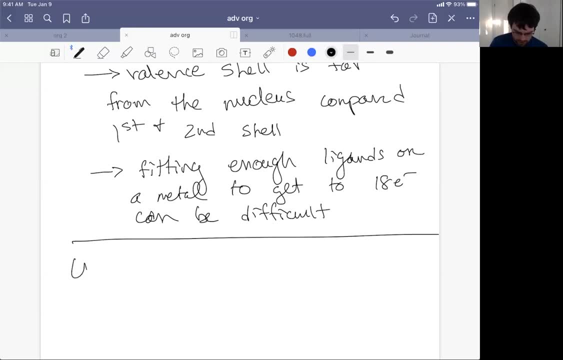 and then compare that number to 18 to see how close we are to a thermodynamically stable metal complex. So using the 18 electron rule is fairly simple. You just. it just takes a little bit of practice to get good at counting where all the electrons come from. But using the 18 electron 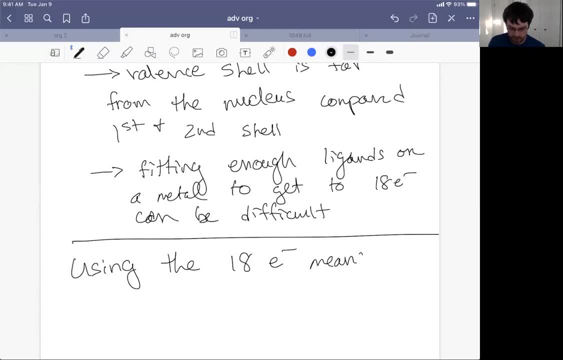 rule means what we have to do is count the number of valence electrons in the complex. Now this in that list of things I said, where I said total electron count, oxidation state and electron count, this is the total electron count, the total number of valence electrons. 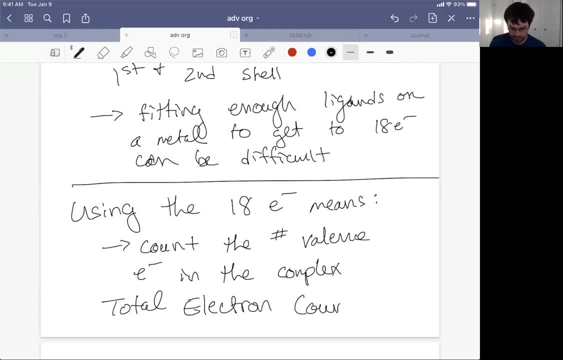 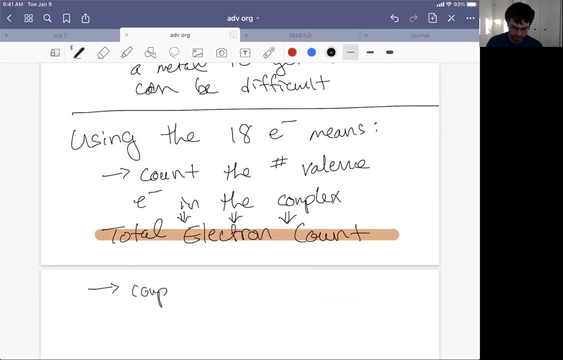 So there's my total electron count, which is again the number of valence electrons in the complex, And what we do is we compare the total electron count to the number 18.. Okay, So we compare it to 18.. And then, if it's less than 18,, we're not yet to like a fully stable. 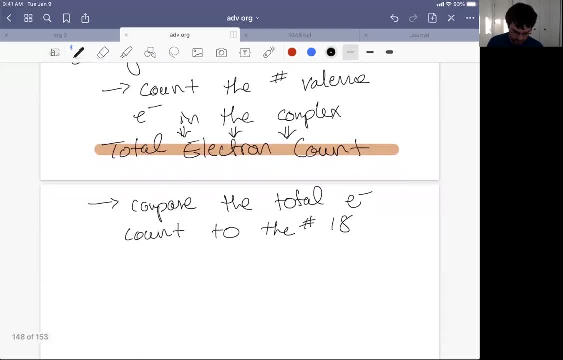 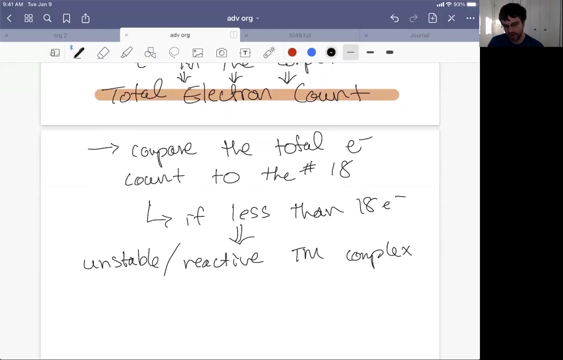 complex. If less than 18 electrons, we probably have a reactive transition metal complex. Now I could write unstable out here. Now the thing that I want to emphasize here is, if we compare, that this is, this isn't like the final molecule We're used to so often drawing the final.